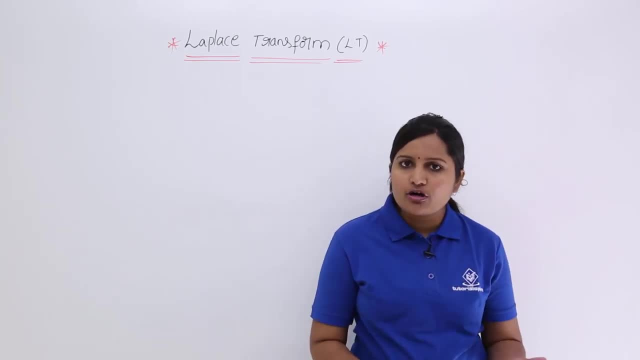 here I will show you what is the advantage of taking Laplace transform. while we consider Laplace transform, even though we are having already one tool to represent any signal in frequency domain, while we came for this new transforms, Laplace transforms. I will show you in the next step itself. 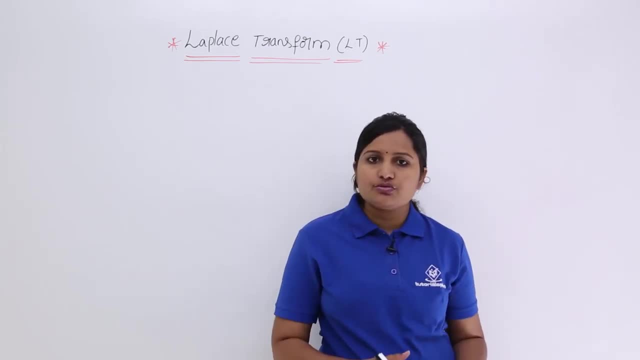 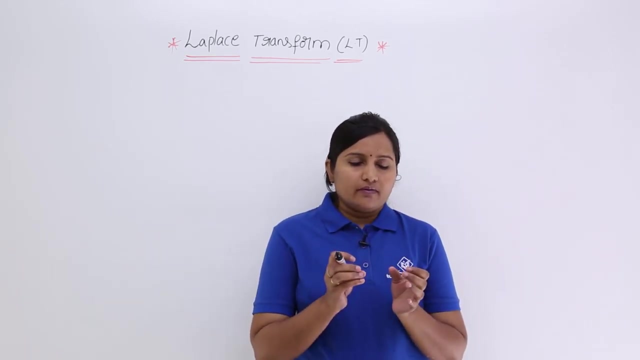 So here I will discuss with you something before getting into the derivation of laplace transformation, to get the equation of Laplace transform. So here AHL is complex. Fourier transform is similar to bilateral Laplace transform. first we need to do one thing, that is, if you you given with a signal, you are given with a signal. and if you are ask: good. 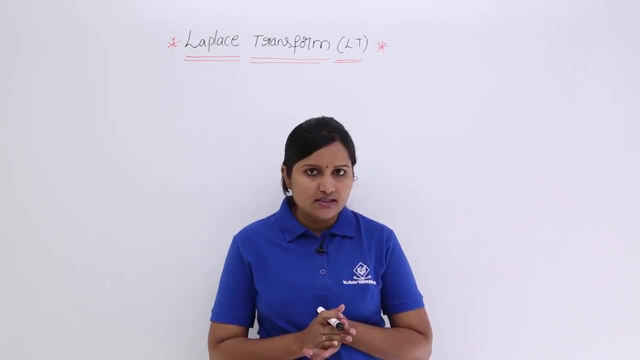 to find out what is the spectrum of that signal. Definitely you need to go for quart root. So if you are given that signal you are asking to find, So if you are given that, So securing you know what the wouldn't be going away, because what are they doing and how can's it doing? 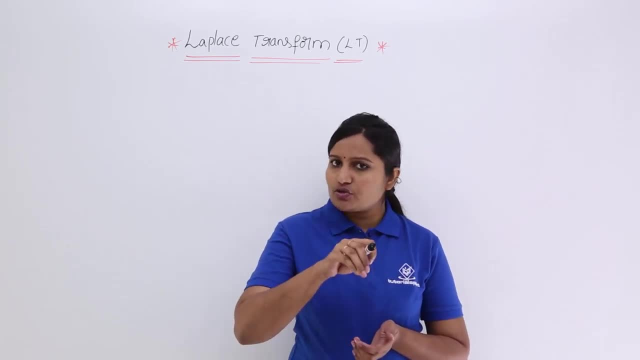 you have different moves to find. If you are given those, what is the spectrum of that signal? definitely you need to go for thought: what is Fourier transform? If Fourier transform is not applicable, then definitely you can't get there is no spectrum for that signal without checking Laplace transform. this is the main. 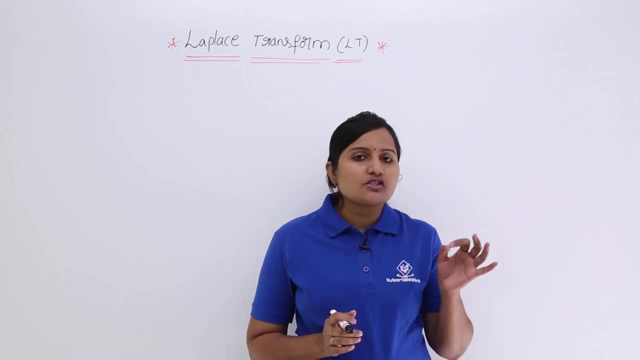 thing: If you are given with a signal and if you are asked to find out the spectrum of the signal for that, firstly, if you calculated Fourier transform, if Fourier transform is not occurring, then that step itself you can't say there is no spectrum for that signal definitely. 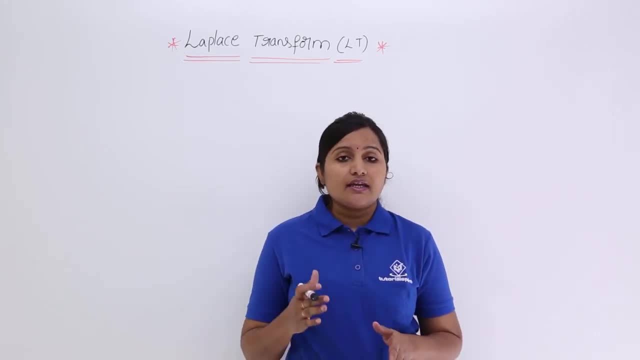 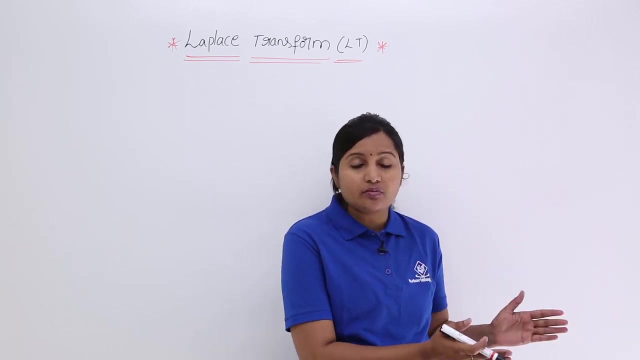 you need to check for Laplace transform of the signal. If Laplace transform is also not occurring, then you can say there is no frequency domain representation for the signal. Otherwise, for so many signals which are not having Fourier transform, they are having Laplace transform. 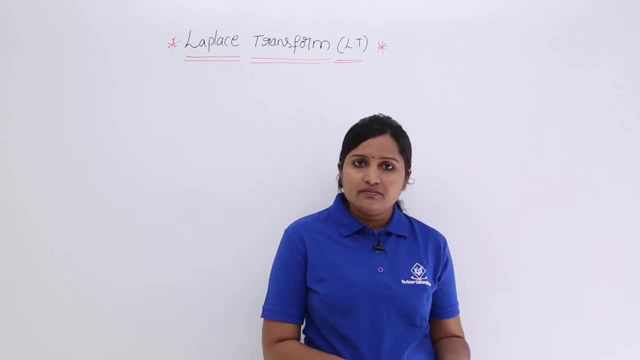 That means if you are having any signal which is not occurring, then you can say there is no signal which is not having which we can't represent in frequency domain by using Fourier transform. there are so many possibilities that we can represent in frequency domain by using Laplace transform. So this is the main advantage of Laplace transform definitely. 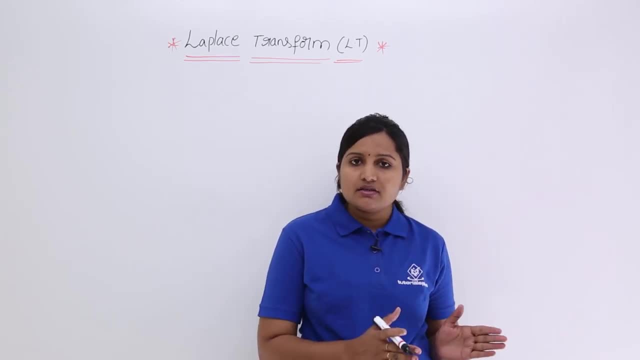 here, whatever the continuous signals which are not having Fourier transform, we can try in Laplace transform. Similarly, if you are having any signal which is having any discrete signals which are not having Fourier transform, we can check z transform. Discrete time Fourier transform. complex discrete time Fourier transform is similar to z transform. 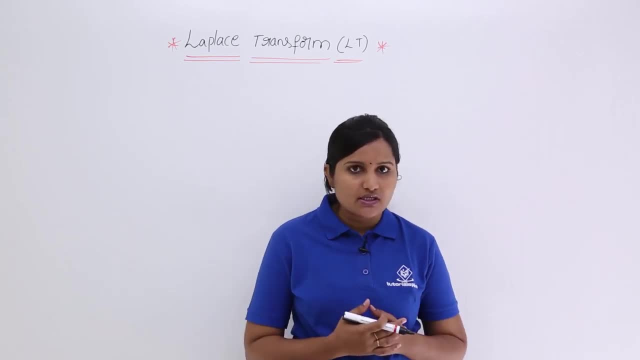 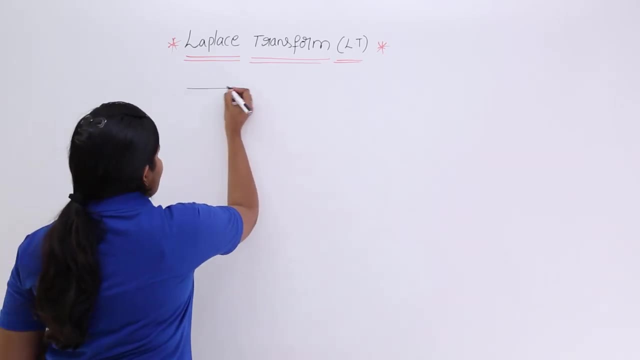 continuous time. Fourier transform is similar to Laplace transform. So here I am considering a signal, I am considering an LTI system. first of all, I am considering linear time, invariant time. It means that I am considering a linear time, invariant time. 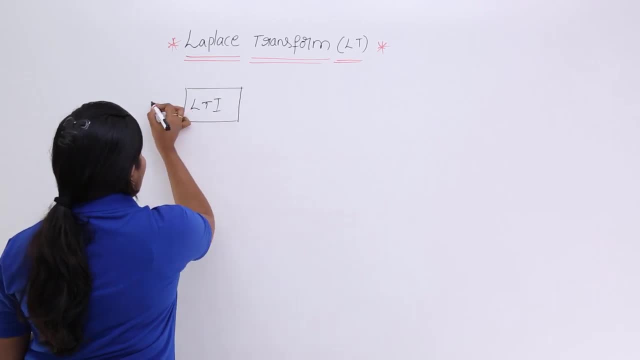 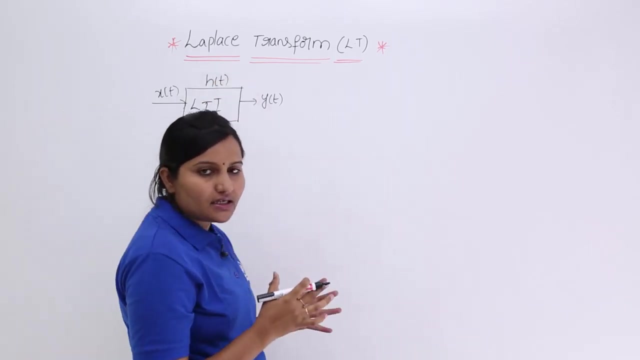 so on and so on From there. on the other hand, I have a state of law where we require linear system. For this system I am giving a signal. that signal is X of t and my output is Y of t. output of LTI system is Y of t and impulse response of the system is H of t. I considered 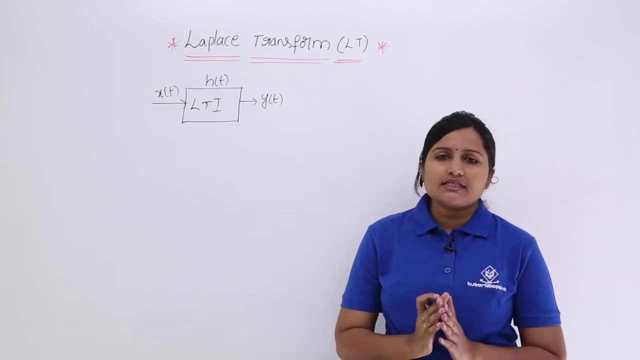 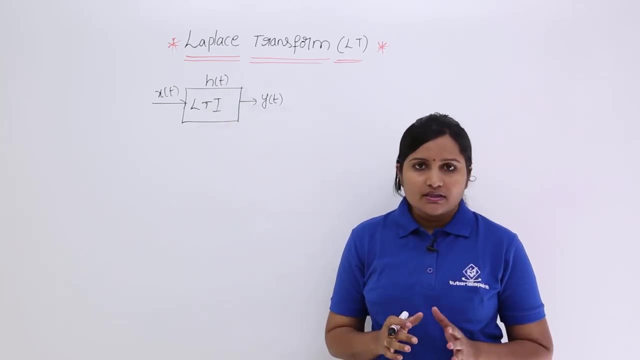 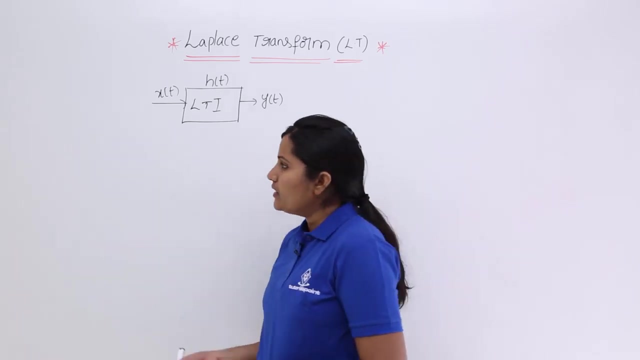 an LTI system. that LTI system is excited with X of t and it is having response Y of t and impulse response as H of t. This type of characteristics that LTI system is having I consider that type of system. So if I am exciting with a complex exponential, 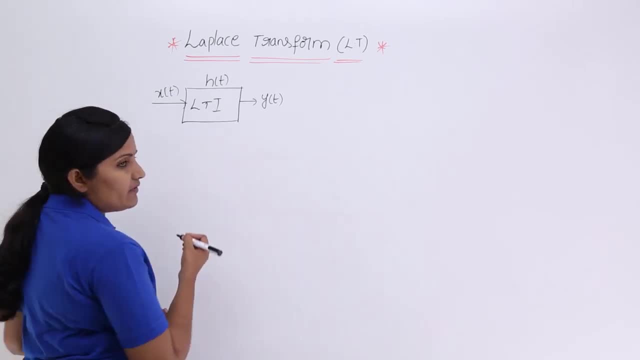 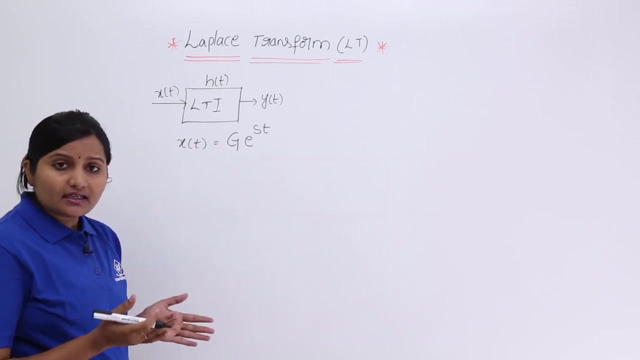 for example, if I am exciting with E power ST, then what will happen? So here, if I am exciting, my LTI system with X of t is equivalent to G into E power ST. So G into E power ST is a complex exponential signal that we are giving as a input to the 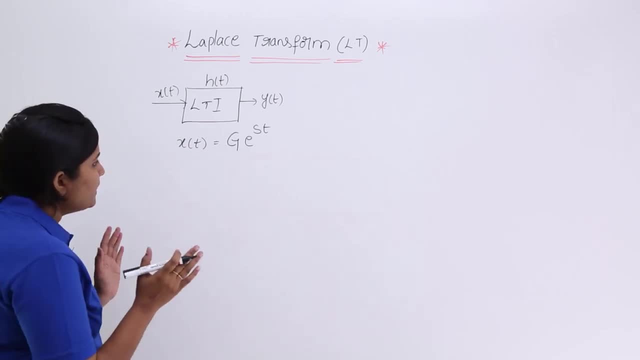 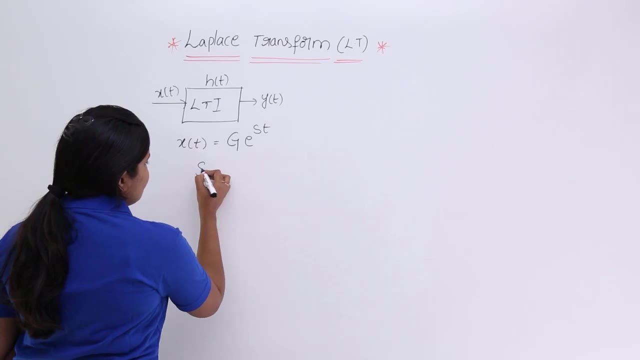 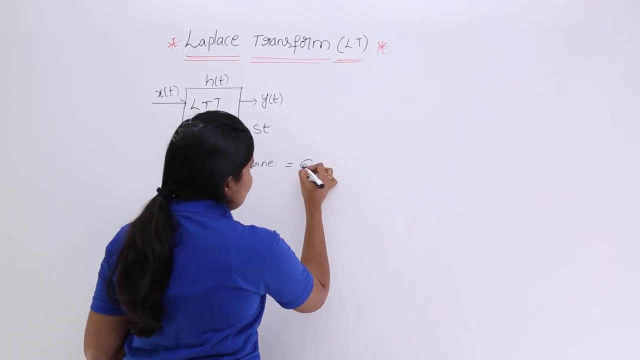 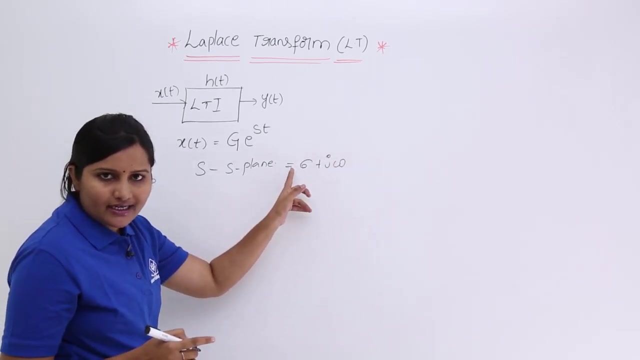 LTI system, Then what will happens? So here, before getting into the procedure, I want to discuss with S. S is nothing but S plane, So where? so S is equivalent to S plane. that is nothing but sigma plus j, omega. Now, previously we covered only omega domain, not real domain, only imaginary domain. we 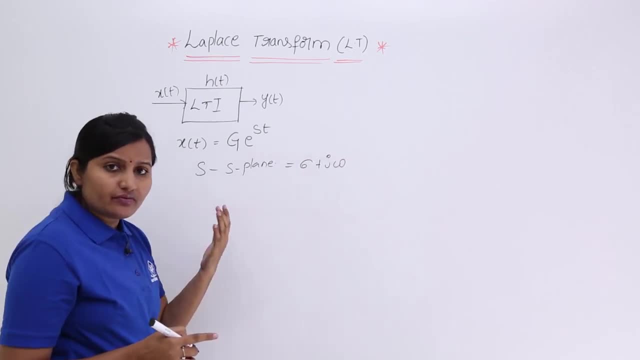 calculated in Fourier transforms Always we are having E, power, j, omega, t, like that. So. but here we are taking all S domain. S domain means real plane plus imaginary plane is nothing but S plane In Fourier transforms. we are having only imaginary plane. we are not having. 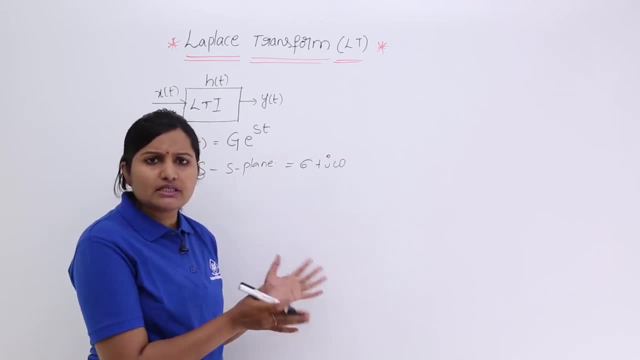 any imaginary plane. So here we are talking about a real plane and the S plane we are any real plane. So some sort of features are going to miss in Fourier transform. that is why if your signal is not having any Fourier transform, please check Laplace transform of the signal to. 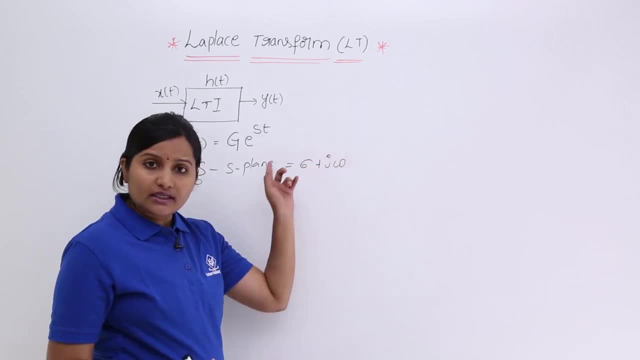 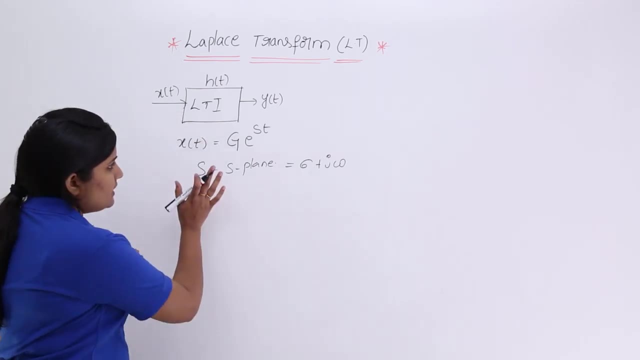 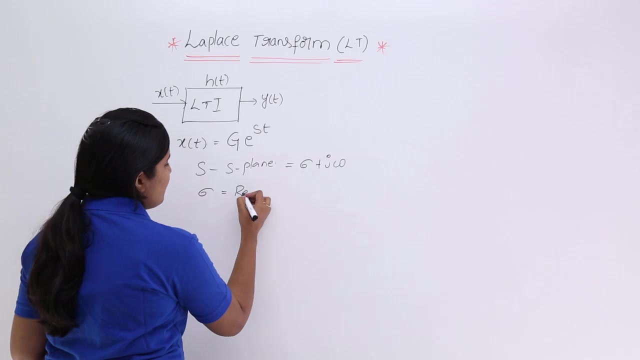 get the spectrum As it is, having both real and imaginary planes, this may give spectrum representation of that signal. So here S is nothing but S plane, which is equivalent to sigma plus j, omega, where sigma is equivalent to real of S and omega is equivalent to imaginary of S. 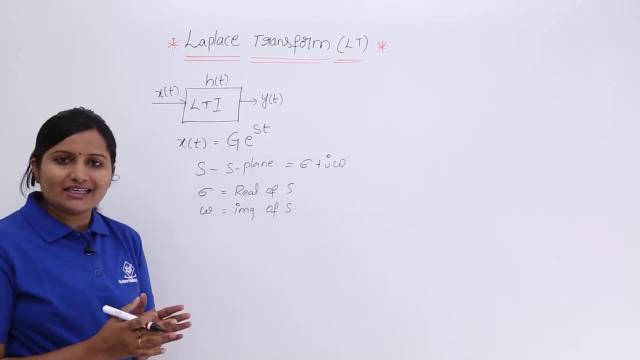 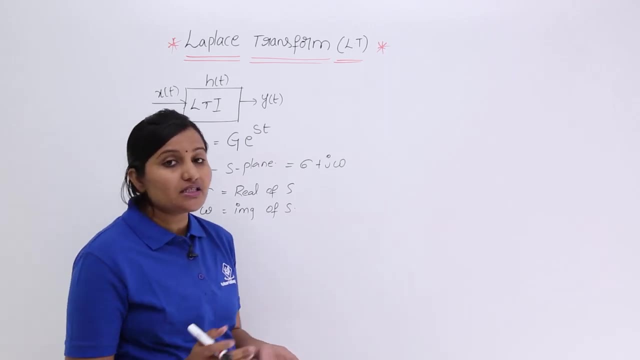 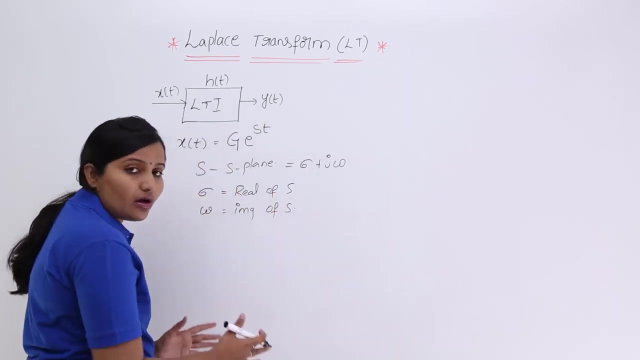 So now I am going into the procedure to get the equation for Laplace transform. So always people will tell you what is. the Laplace transform means integral minus infinity to infinity, x of t into e, power minus s, d, dt. how we are getting that formula So that I will derive now. 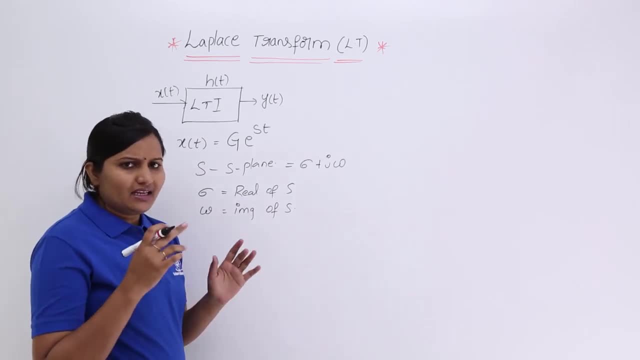 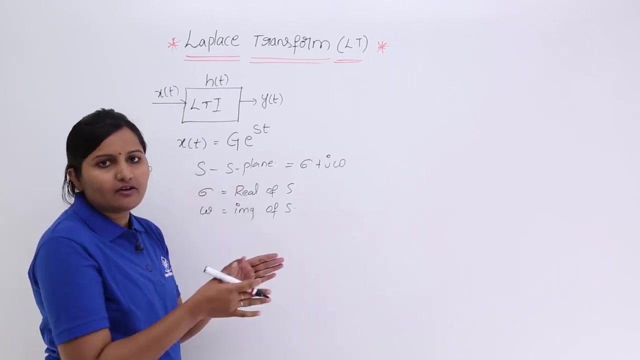 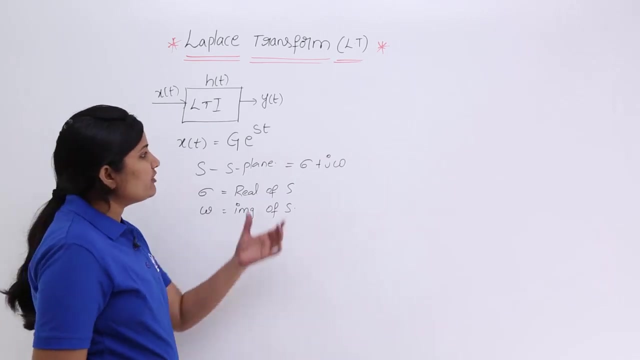 So here, what we are discussing, For any derivation or for any system, we are giving complex exponential. If you are giving complex exponential, that formula can be used for so many signals. that fundamental formula can be used for so many signals. That is why I am giving- I am exciting- my LTI system with a basic signal. 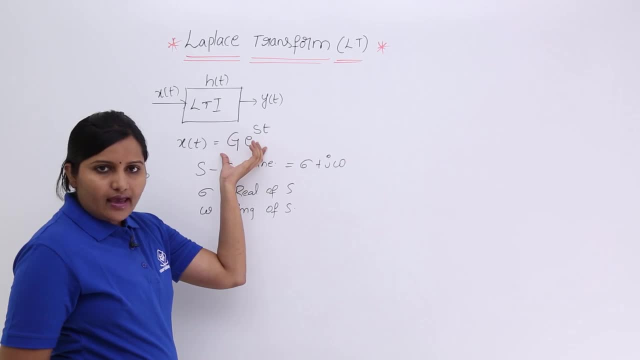 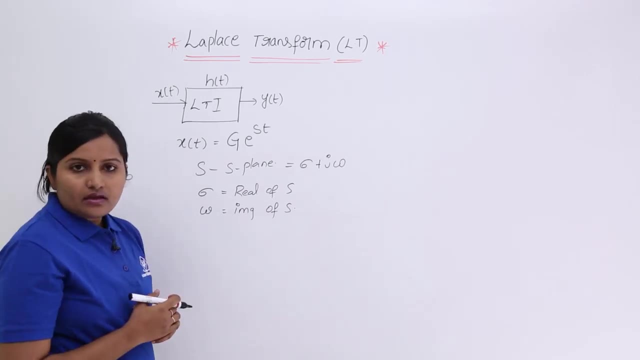 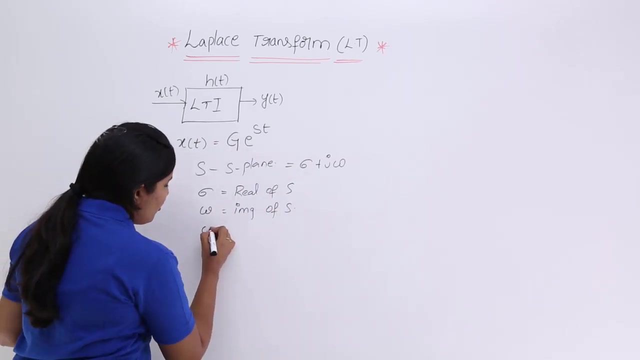 basic complex exponential signal as g into e power st. I have given this signal for my LTI input. So you know that the LTI system will produce output based on its input and impulse response. You know that output of LTI is equivalent to input convolution. 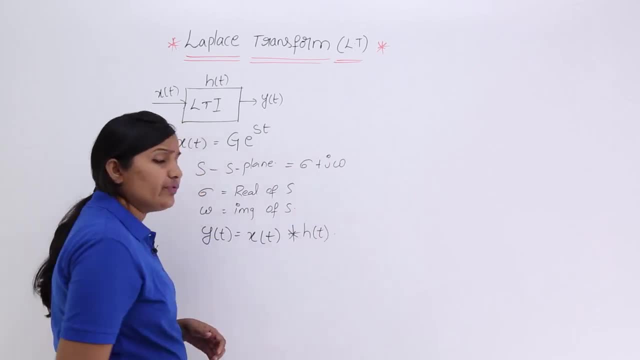 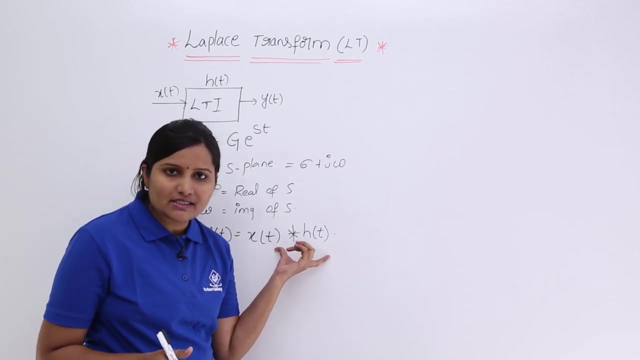 with impulse response. When we are discussing the relation between input, output and impulse response of LTI system- there I discussed always, output of LTI system is equal to input of LTI system. So you know that LTI system is equivalent to input convolution with impulse response. 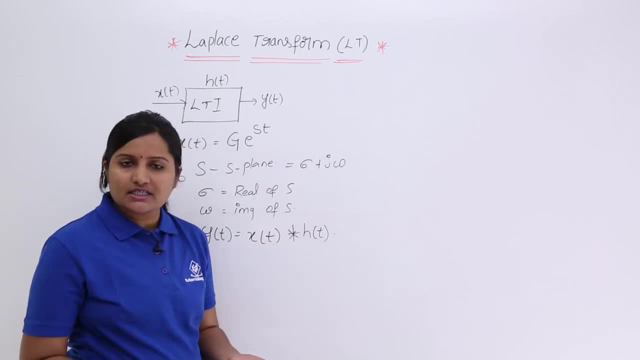 So you know convolution formula. we already completed convolution related videos. also, We are having a formula to calculate x of t convolution with h of t. that formula is equivalent to integral minus infinity to infinity: h of tau, x of t minus tau d tau. this is the 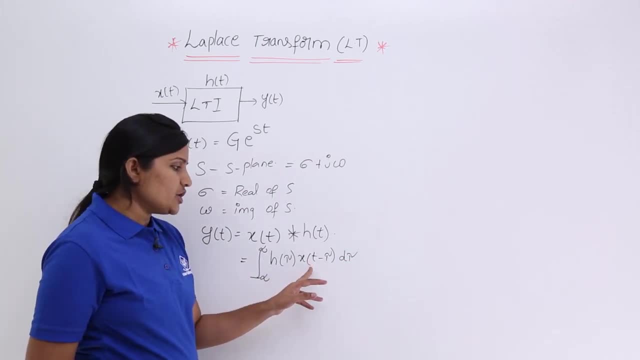 formula. you can write like this also: x of tau, h of t minus tau, d tau. also write like this: You can also write it by using this expression: if you get a formula which can be used in a also, you can write Why I am shifting the signal means I do not know the impulse response of the. 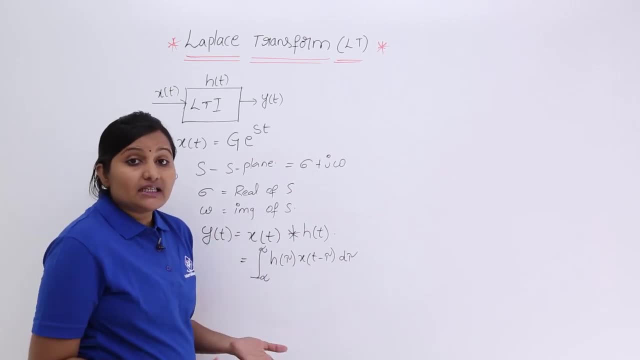 system. I just know with which signal I am exciting the system. I know only the input signal. That is why, whatever changes I want to make in convolution, I am changing on known signal, only This. I do not know anything. That is why I cannot move further. That is why I am using that shifting on my known 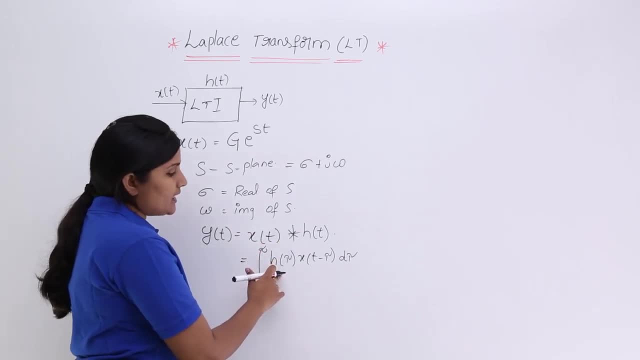 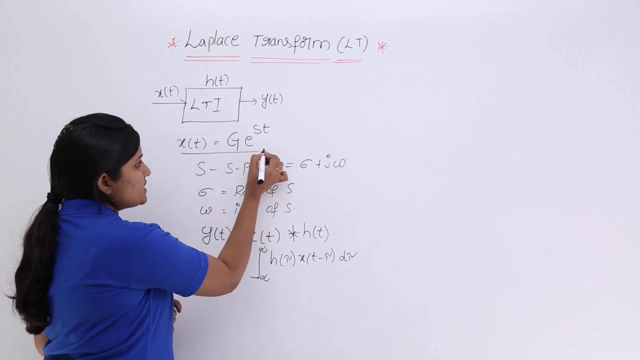 signal. That is only the reason. But here you can write x of tau, h of t minus tau d tau. If you return like that you cannot get next step how you need to follow. So here I consider convolution like this: Here you know x of t, Your signal: x of t, You know x of t. I am just going to substitute. 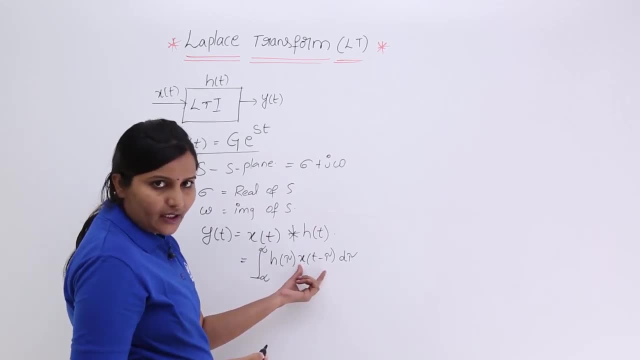 that x of t in place of x of t minus tau. How you will get x of t minus tau if you are having x of t minus tau. You will get x of t minus tau if you are having x of t minus tau. So here you. 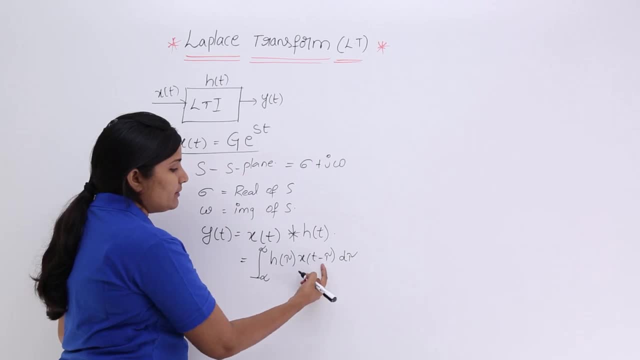 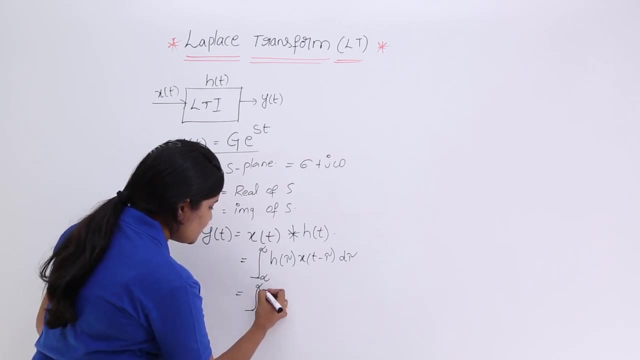 can write x of t means in place of t. if you substitute a t minus tau, So you are going to get x of t minus tau. So that is equivalent to integral minus infinity to infinity h of tau. x of t minus tau, Please. I am just substituting t minus tau in place of t, So g into e power s. 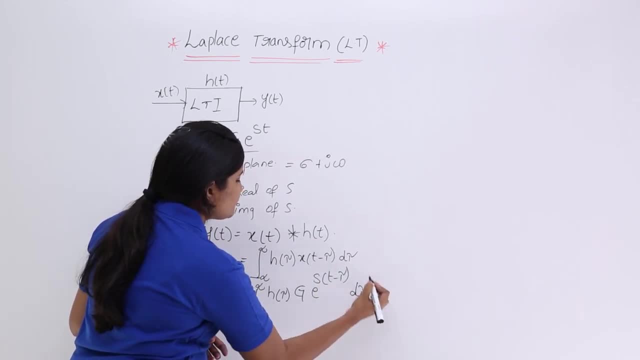 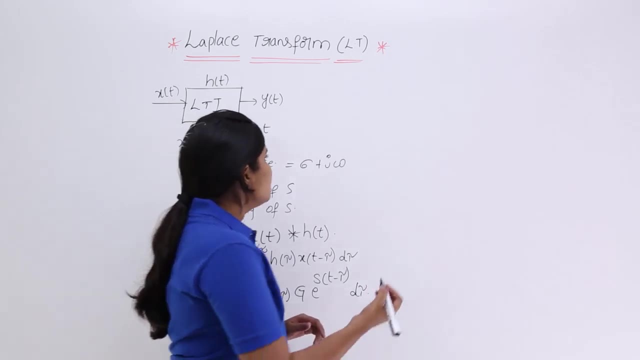 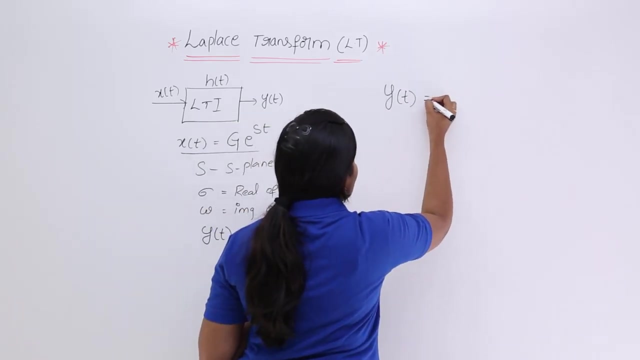 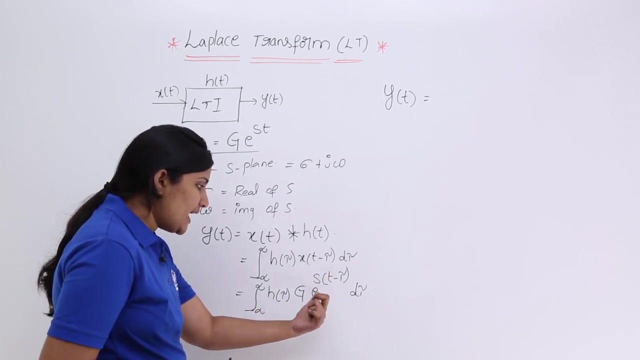 into t minus tau, d tau. This is your modified equation, So now. so finally, this is y of t. We are calculating for y of t. Y of t is equivalent to: here you can see the integration in terms of tau domain. and if you see here, here you are having 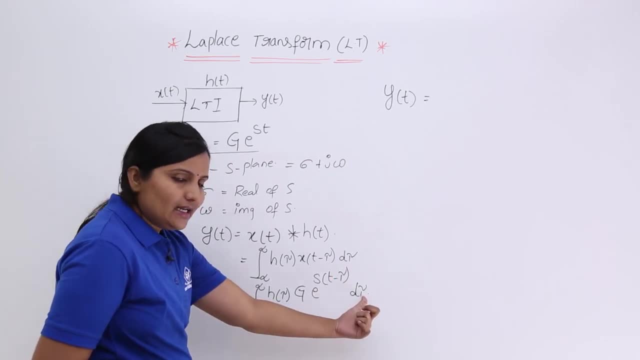 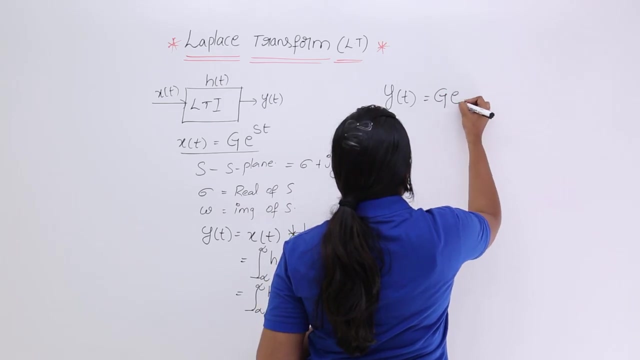 e power s t. If you are calculating your integration in tau domain, e power s t will become the constant, and one more constant is there, that is g. These two I am keeping it out. So here that is equivalent to g, into e power s t, integral minus infinity, to infinity, and 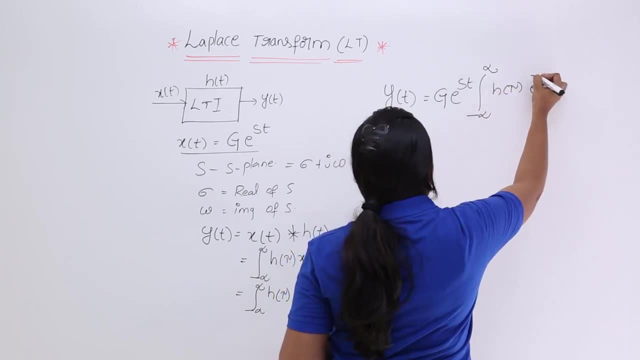 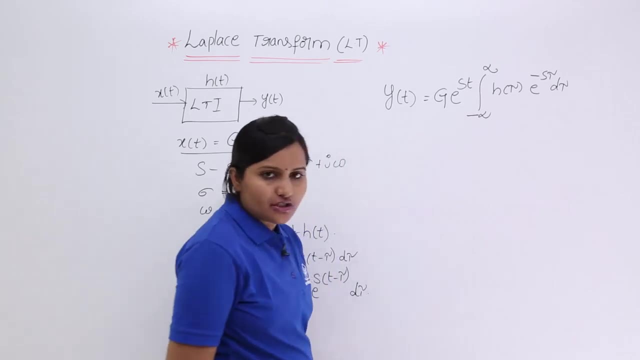 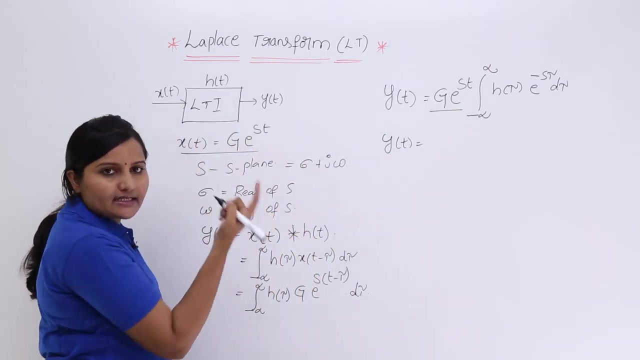 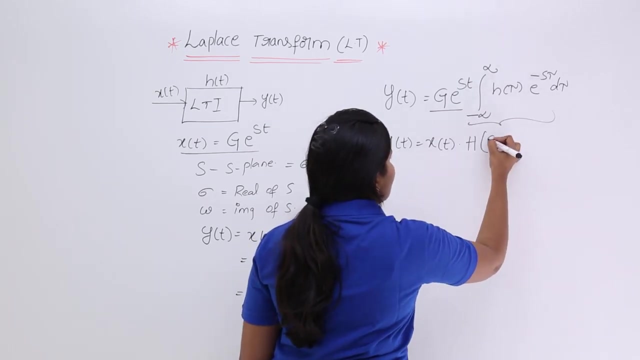 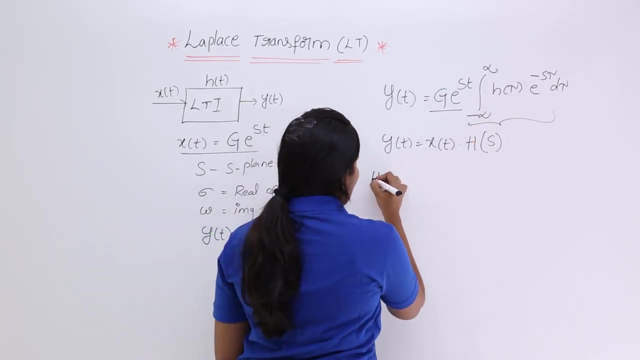 h of tau, e power minus s, tau d tau. So this is the remaining equation. So now here, y of t is equivalent to g. into e power s, t is nothing but x of t. So you are given signal. So x of t into this one I am considering like h of s. Let it be considered as h of s, Where h of s is. 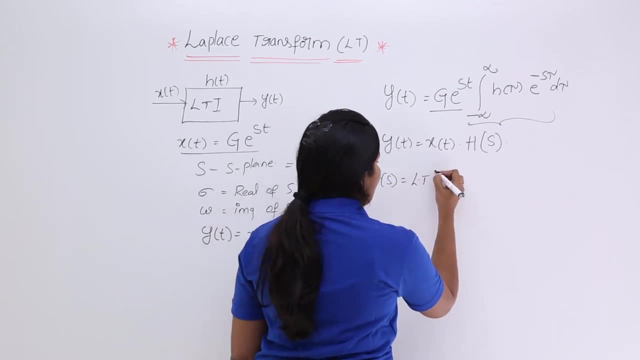 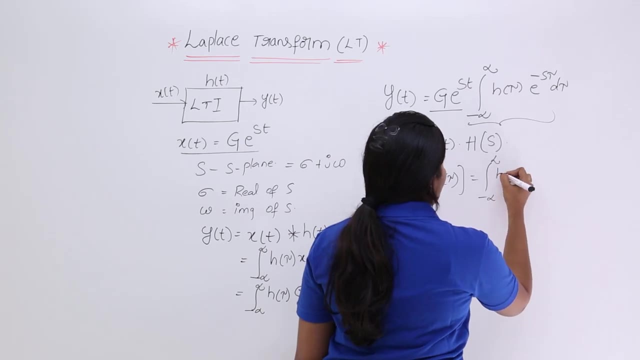 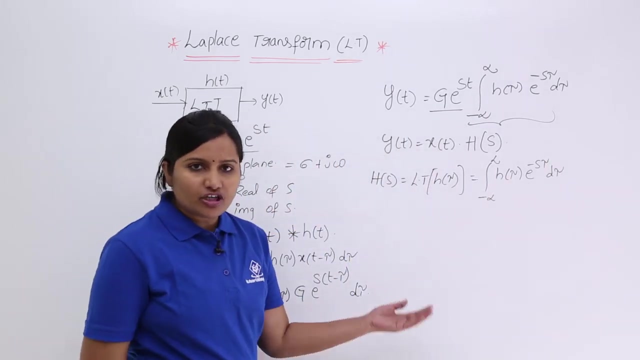 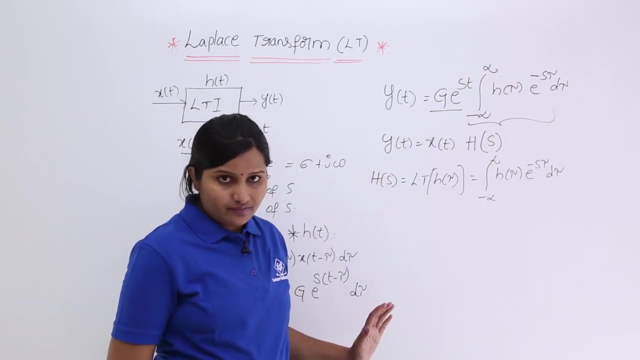 equivalent to Laplace transform of h of tau. So that is equivalent to integral minus infinity, to infinity h of tau, e power minus s tau d tau. If you replace tau with t, then you are going to get Laplace transform equation. So here this is nothing but Laplace transform of the signal. So 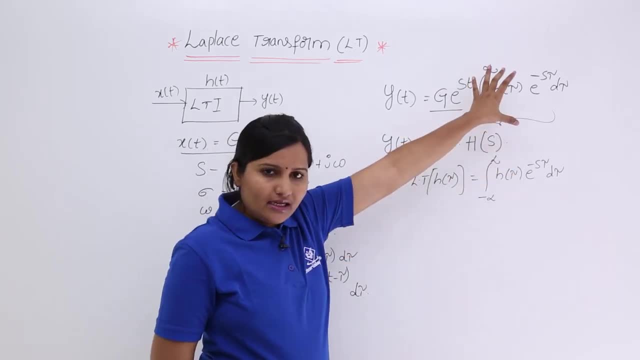 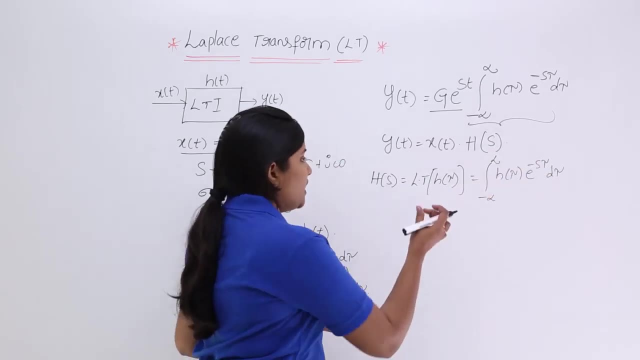 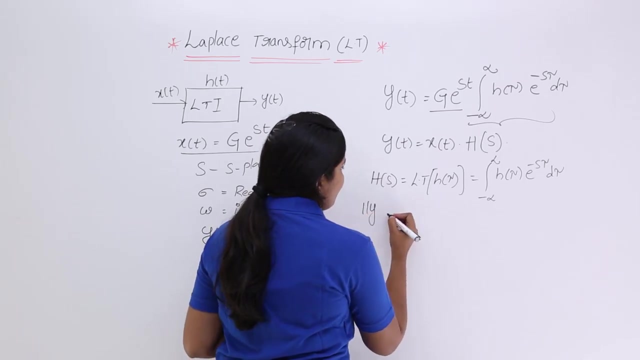 here h of s is equivalent to what I considered h of s. I written that. So that is nothing but Laplace transform of h of tau. That means if you want h of tau Laplace transform, then you need to calculate like this. Similarly, if you want Laplace transform of x of t, then how we will. 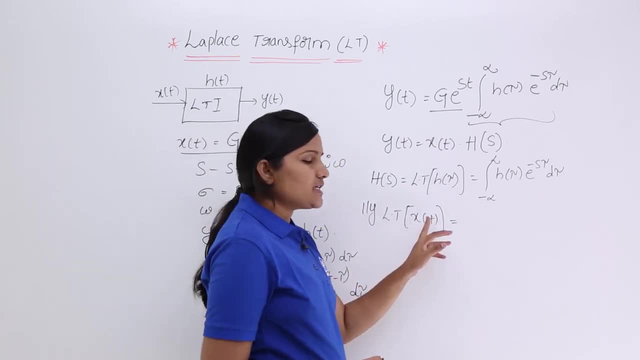 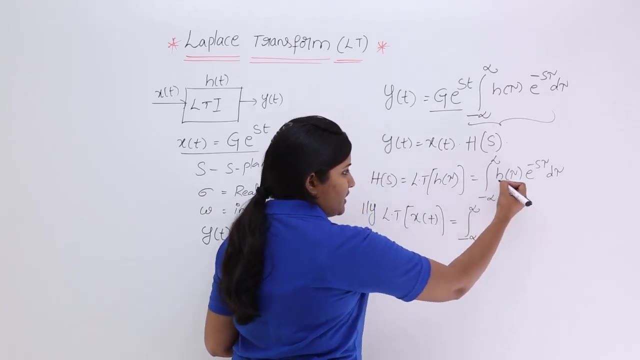 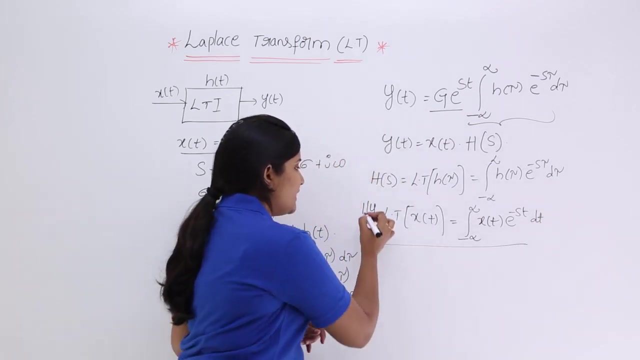 calculate Laplace transform of x of t means: So: Laplace transform of x of t is equivalent to: so integral minus infinity to infinity. I am just following this equation: x of t into e power minus s, t, dt, This is the Laplace transform of x of t. So for any signal x of t, the Laplace. 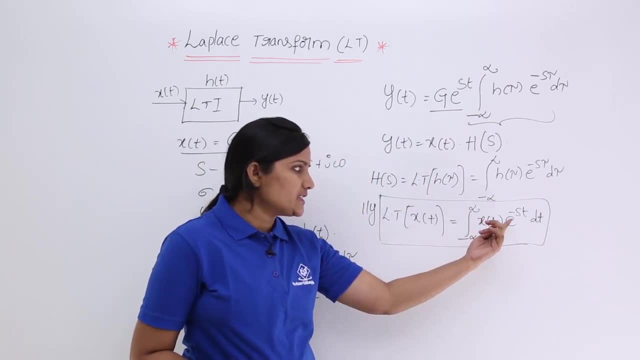 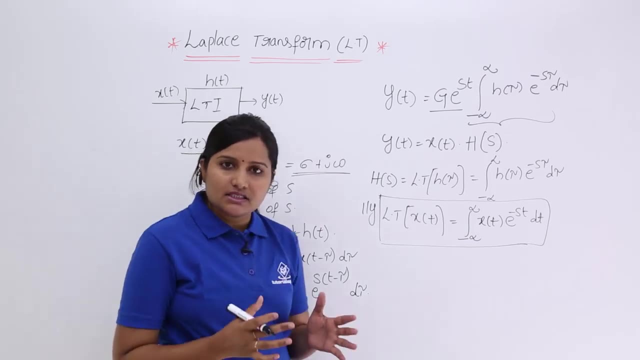 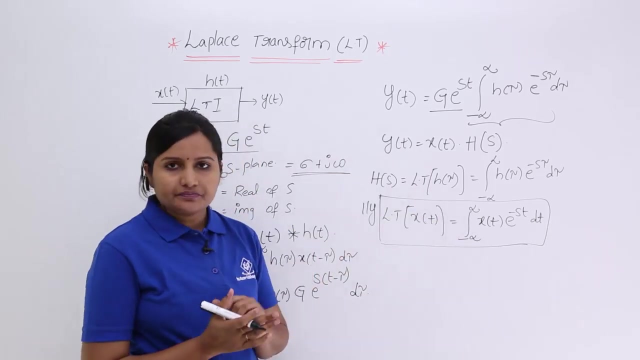 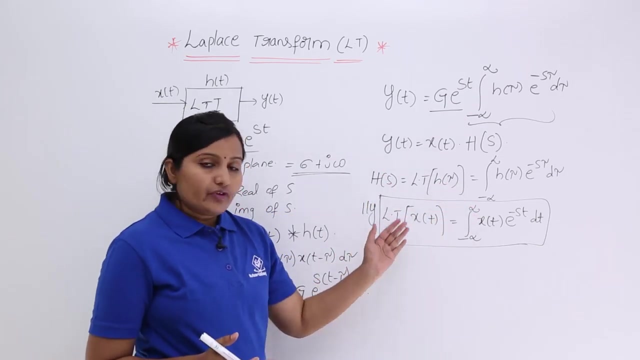 transform is integral minus infinity to infinity. x of t into e power, minus s, t, dt, where s is sigma, plus j, omega, where sigma is the real part of s and omega will be imaginary part of s. And here this is your Laplace transform of your signal. We are having other relations like 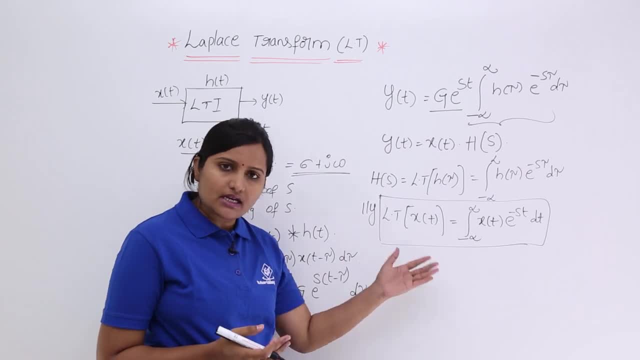 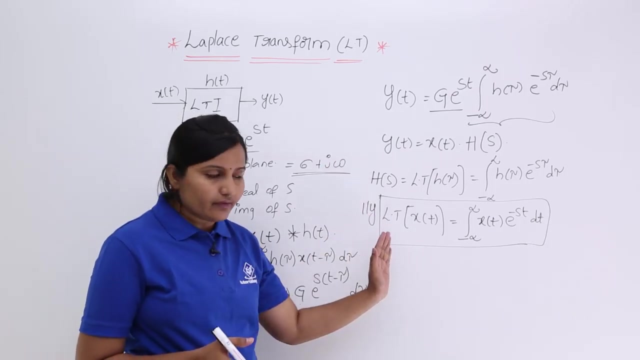 Fourier transform, other relations. this Laplace transform is having relation with Fourier transform and how we will get inverse transform and all these topics we will see in the next class. So in this video we got an idea of Laplace transform, how we got this equation as Laplace. 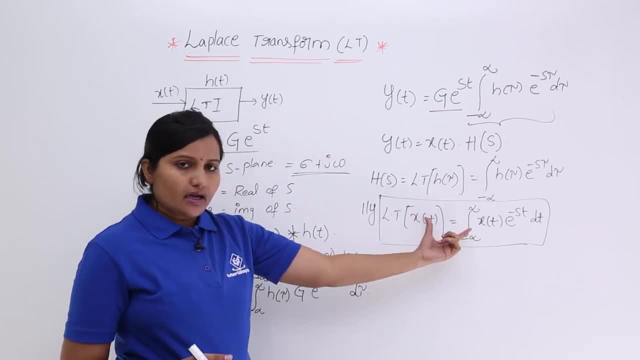 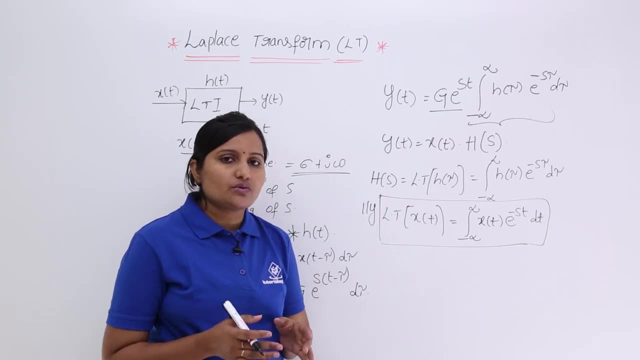 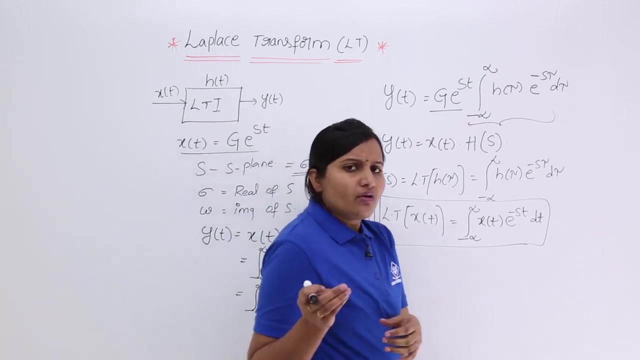 transform equation. So in this video, so I showed you this Laplace transform equation. This is very, very important. So here this formula is going to use for different differential equations, to solve differential equations and etcetera, and etcetera, Definitely, whatever questions related to. 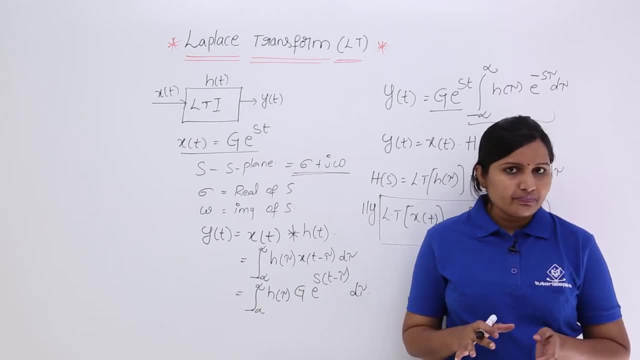 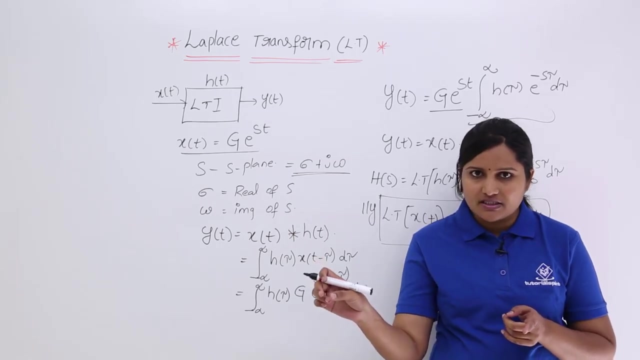 that you are going to solve with Laplace transform only In future. in any exam, if you are getting spectrum, find out the spectrum or anything related to differential equations In the question itself. if you are having differential equations and the question is related to, 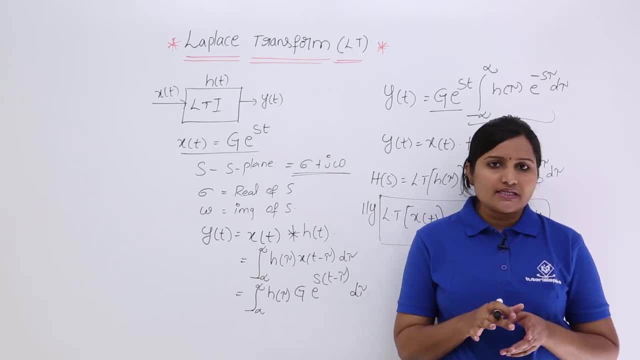 spectrums or anything you are going to solve with Laplace transform. That is easy to solve with Laplace transform. Please keep in mind, when you are solving differential equation related topics related to spectrums or signals. then just go for Laplace transform. that will provide better. 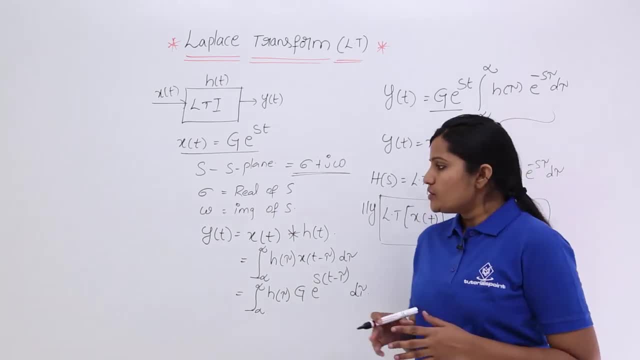 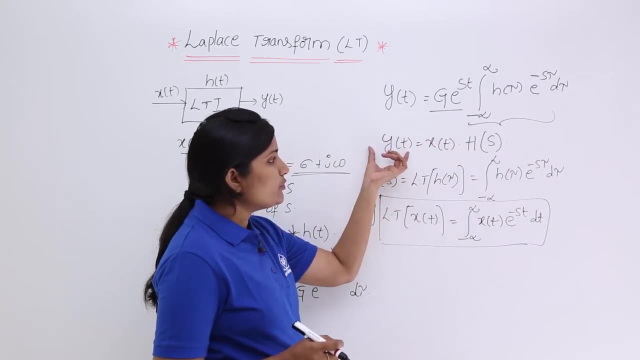 solution within minimum amount of time. So here, coming to the relation between Laplace and transfer function and output is: if you consider h of s is equivalent to, h of s is equivalent to y of t by x of t, that is equivalent always your transfer function, h of s is equivalent. 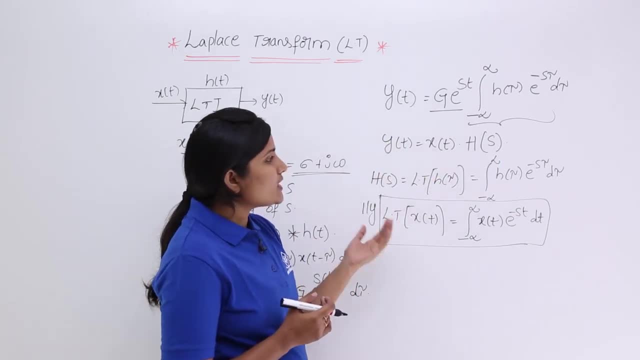 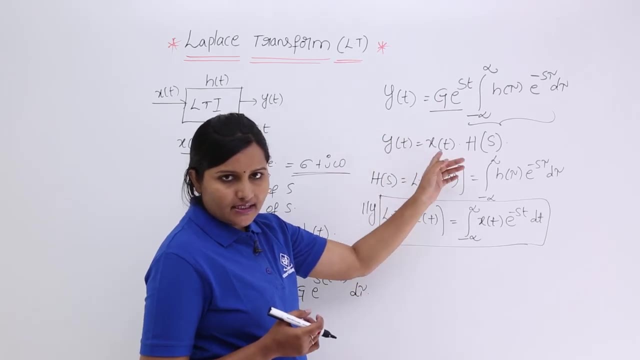 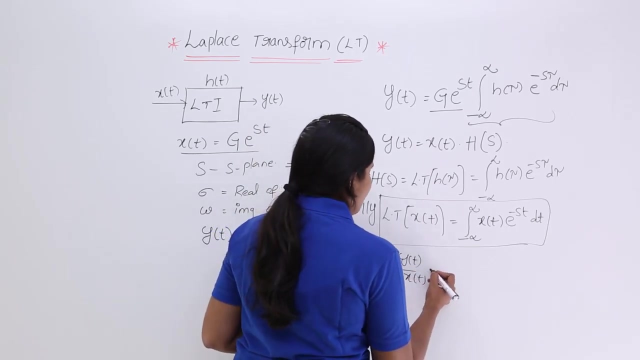 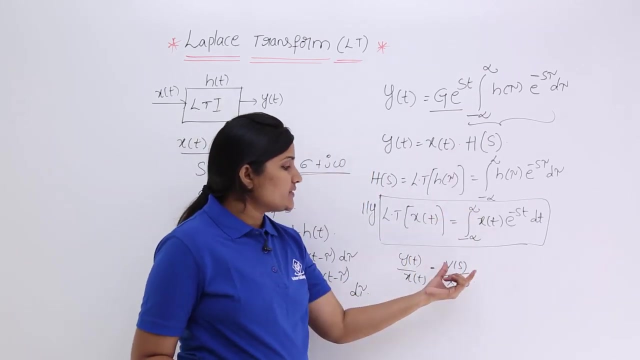 y of t by x of t, if you consider transform. So if you consider transform of these 2, y of t by x of t, then you are getting the same ratio. that means y of t by x of t is equivalent to y of s by x of s, y of s by x of s. I will show you how we will get this. So h of s. 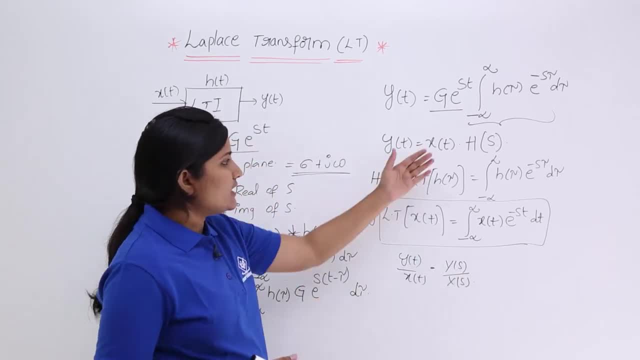 we can say y of s by h of s. like this: we will get h of s by h of s. So if you leave S 1 by H of S, you will get h of S into 1 by H of S, into N of S, by N of S, into apply. 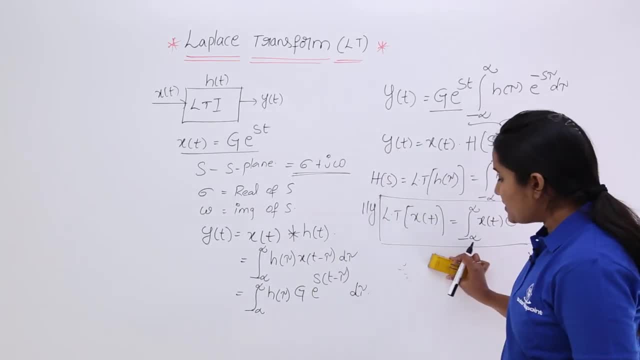 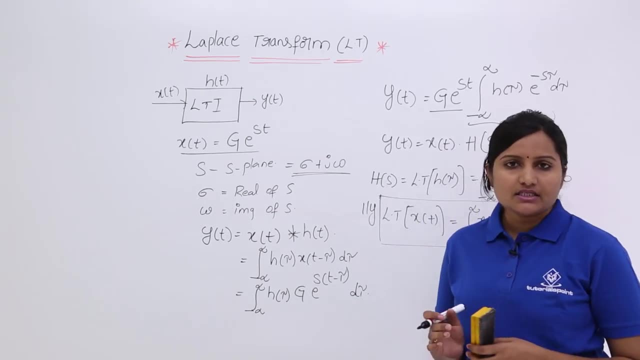 How many types of problems will get on this? Laplace transform means they will ask: what is the Laplace transform of the signal? by using this equation we can found the Laplace transform of the signal. For example, if they given transform of the signal and if they